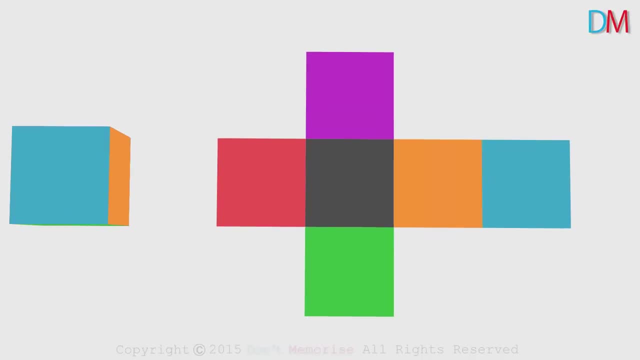 If we look at it from the top, it will look like this: The orange face is the face to the right, The blue face is the top face, The green face is the face in the front, The black face is the base. The purple one was on the one at the back. 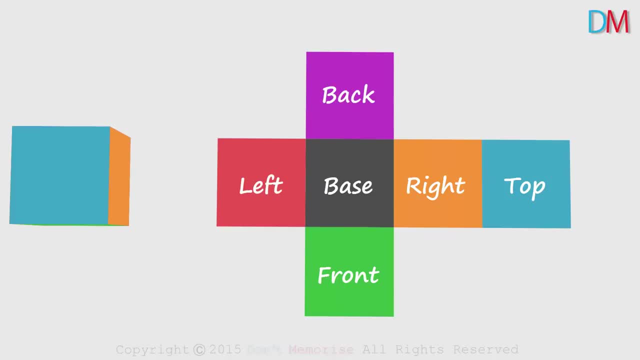 And the red one was on the left. Yes, all we did was open up the faces along the edges and we got the net of a solid. Now listen to the next question carefully. Does the net of this solid have to look exactly like this? 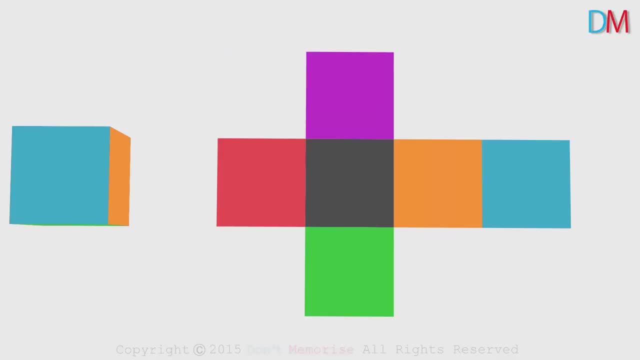 Is this the only possible net of the cube? Maybe not. Let's see if we can open up the same cube differently. We open up the top face first along this edge, Then we open up the front face outwards, Then we open up the top face first along this edge. 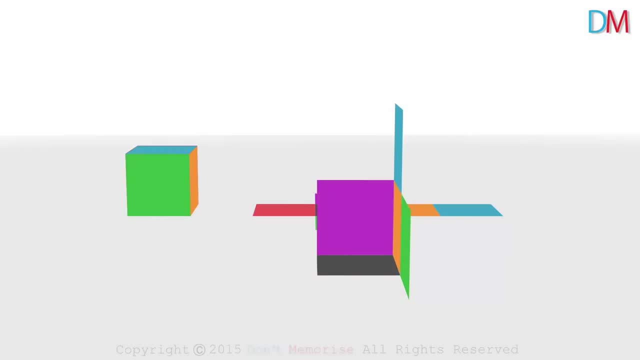 Then we open up the front face outwards, Towards the right, Then we make the side face fall towards the right. There are still two faces remaining, The purple one at the back and the red one to the left. So we drop the left face towards the left and the back face backwards. 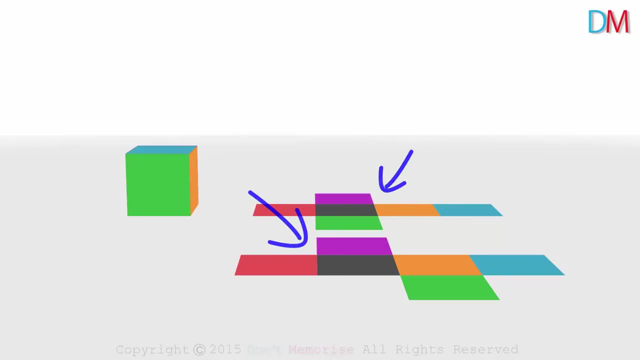 This is what we get. It's clearly different from the earlier one. To know how it's different, let's look at the top view. The top view will look like this, So drawing the net of a solid may result in different figures. 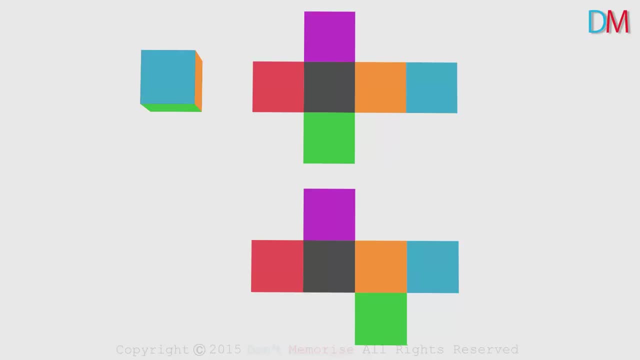 It doesn't have to be the same. I'm sure you have understood the concept of a net by now. It's easy for me to draw the net of a three-dimensional shape using software, But how would you draw the net of a solid in your notebook? 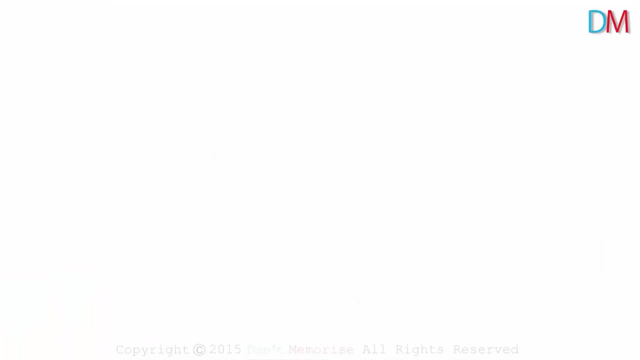 Well, you would have to pull out the architect in you. Look at this cube. How would you draw the net of this cube in your notebook? You don't have 3D software, So you need to imagine 1. One good way to draw a net would be by naming the faces. 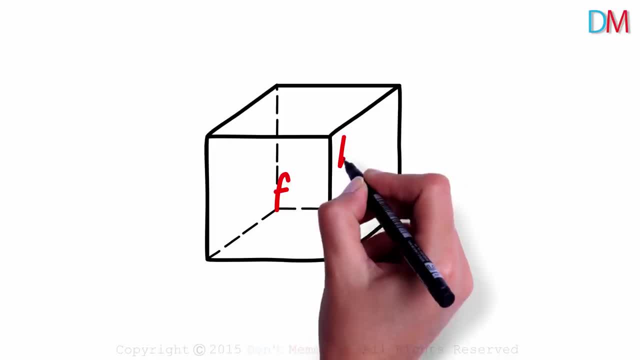 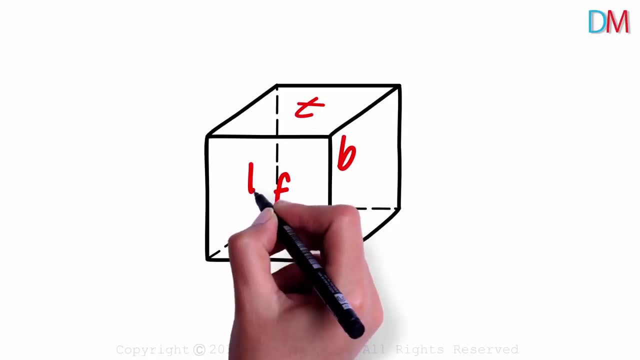 We can call the face in the front F and the face at the back B. The face which is down can be called D and the one at the top can be called T And L and R for left and right. These are the six faces.